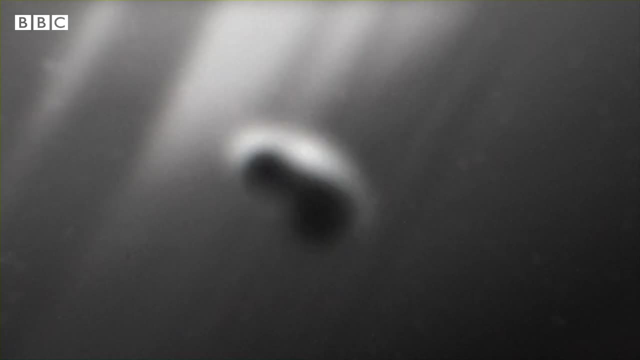 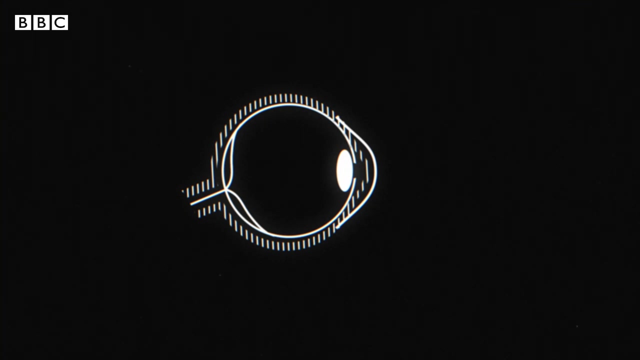 sun emits the most of. Given our early ancestors lived in the sea and were illuminated by the sun, it makes sense that we would evolve to detect the most common and useful wavelengths in the EM spectrum. Our eyes detect colour via specialised cone cells. There are three types of cone cell. 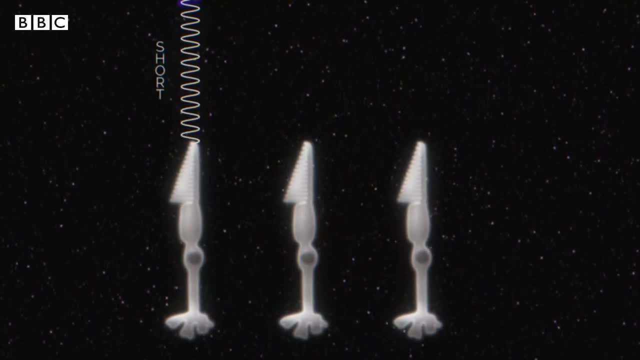 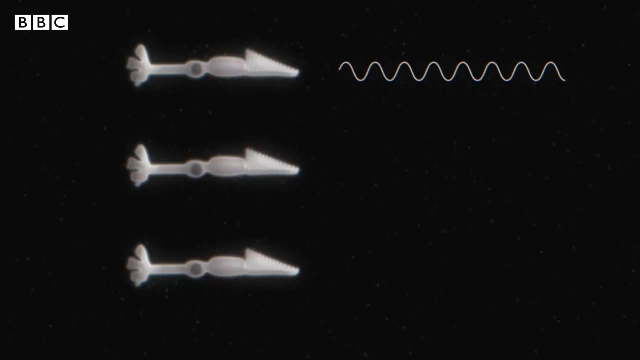 in the human eye: Ones to detect short wavelengths- the blues. one to detect medium wavelengths- the greens, and one to detect long wavelengths. Ones to detect long wavelengths- the reds. But we see more than just red, green and blue. 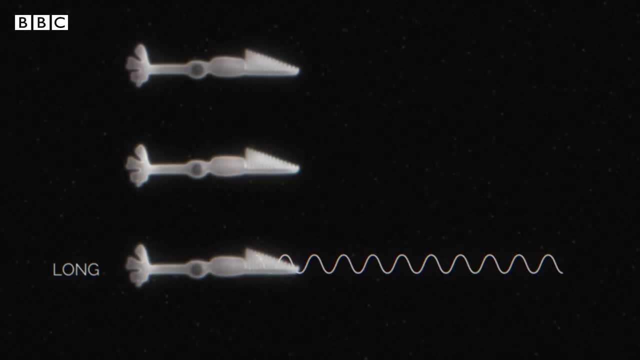 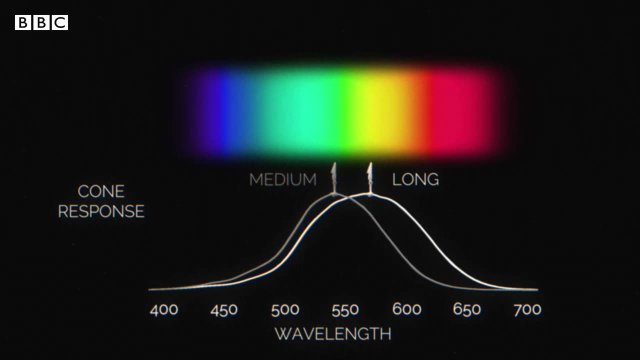 The cone cells in your eyes overlap in the wavelengths they detect. Look at this chart. You can see that when a ray of light with a wavelength of 570 nanometres enters your eye, it stimulates both the long and medium cones. Their responses are combined. 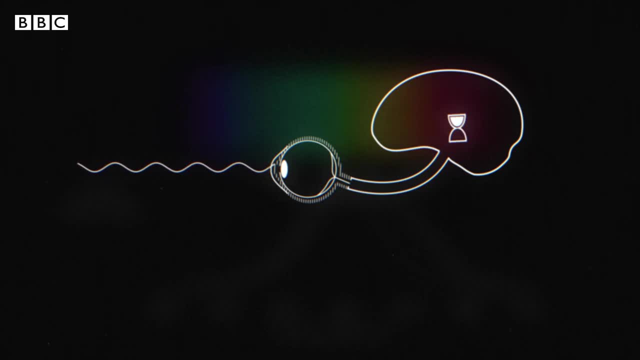 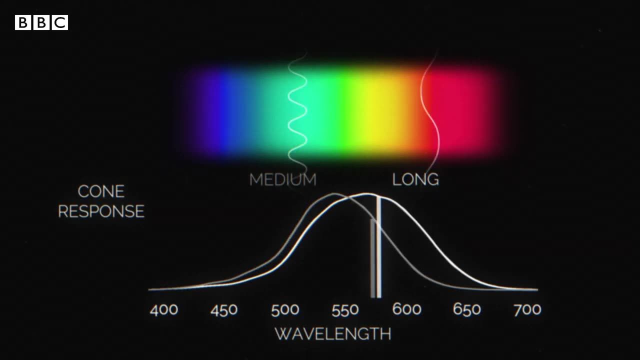 and sent along the optic nerve as one signal, And it's this signal that we interpret as yellow light. An odd quirk of this system is that when two beams of light at the exact same ratio enter the eye, the signal that is sent off to the brain is the same. 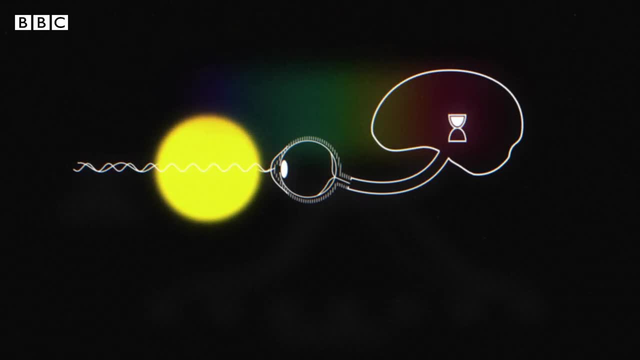 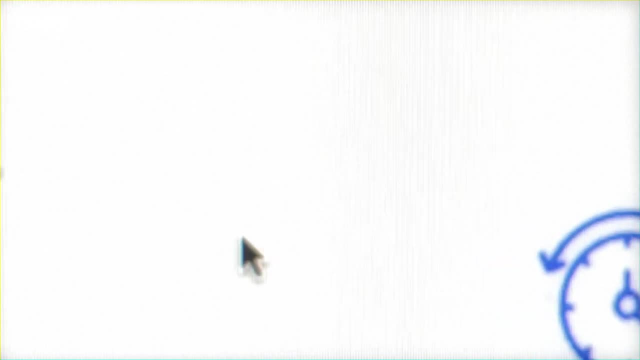 These two combined light rays also cause us to see yellow. The screen that you are watching this on takes advantage of the way our brain perceives colour. If you look closely, you can see that screens are composed of small clusters of just red, green and blue lights. 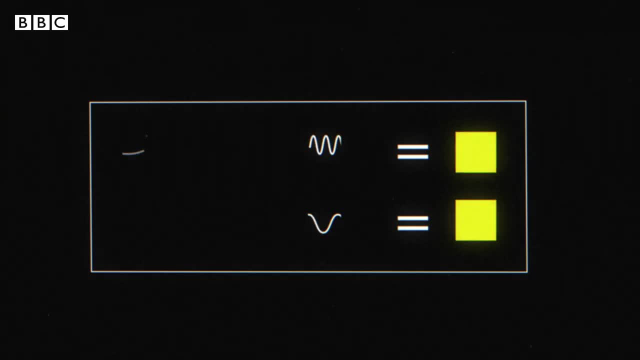 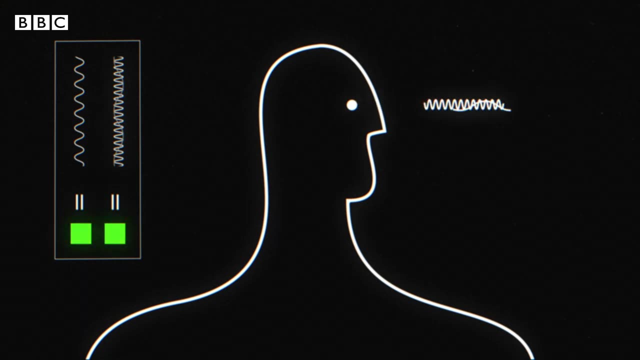 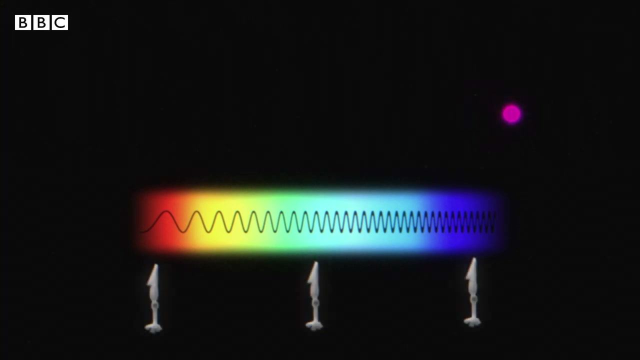 Yet your display can produce the whole spectrum. Every colour that we perceive can be generated via this dual route: a single wavelength of light or a combination of wavelengths that stimulate our cones in the same manner, Except one: Magenta. There is no wavelength of light for magenta. 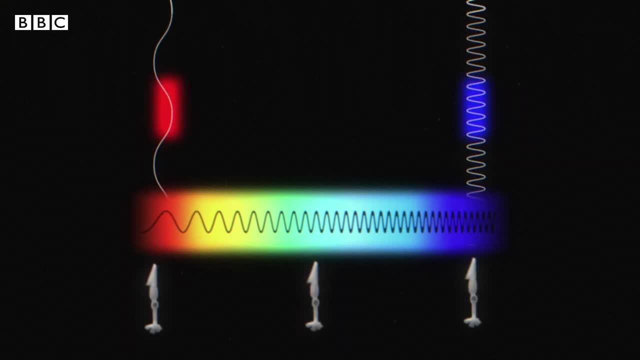 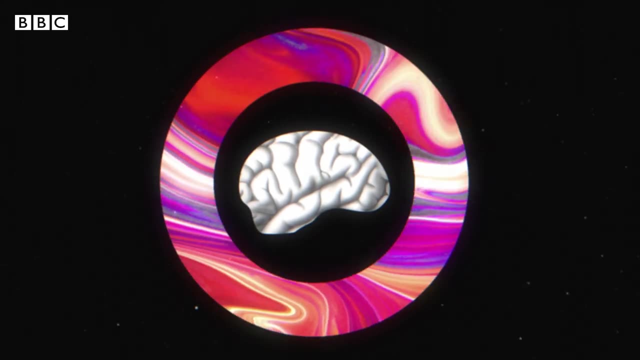 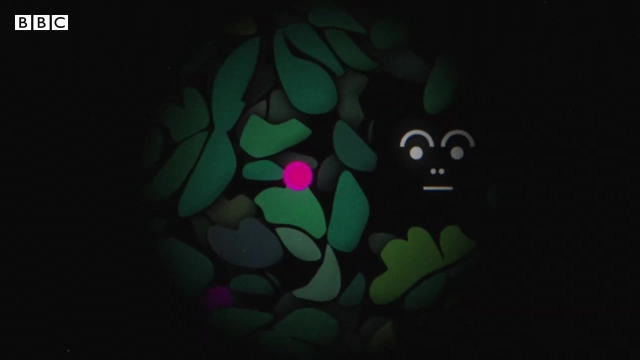 Instead, we perceive it only when the S-cones and L-cones pick up a signal from pure red and blue light, Our brains literally make up magenta. Why, We don't know. It's probably quite useful, though, given that much of our early primate ancestors were in